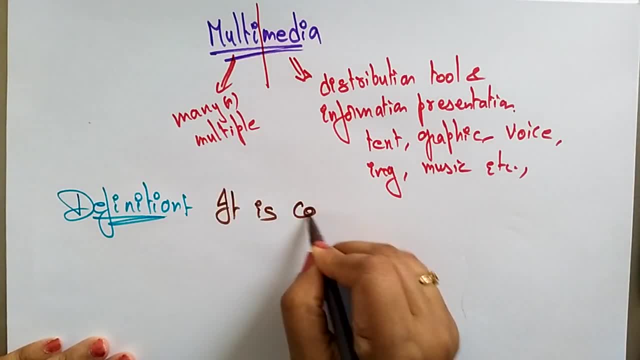 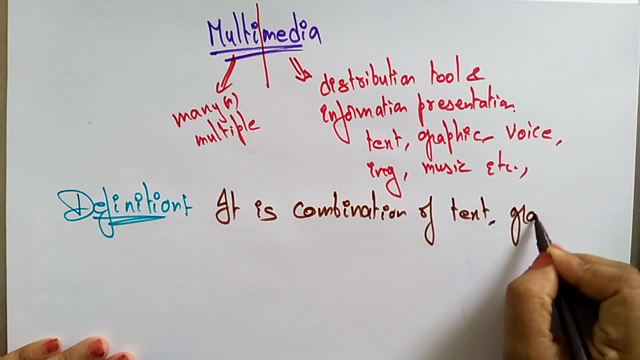 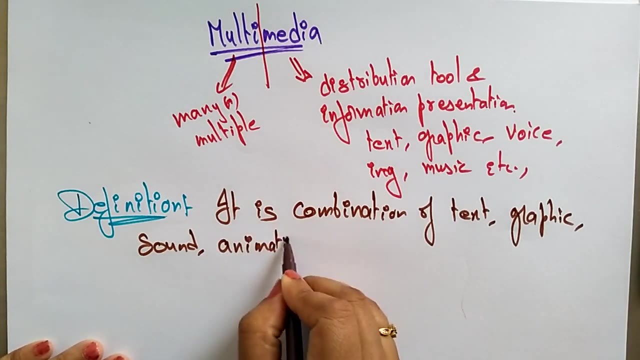 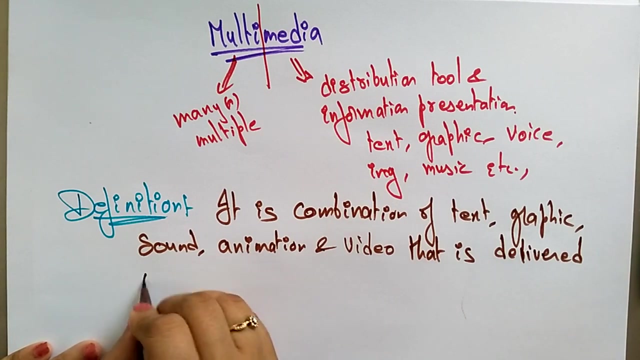 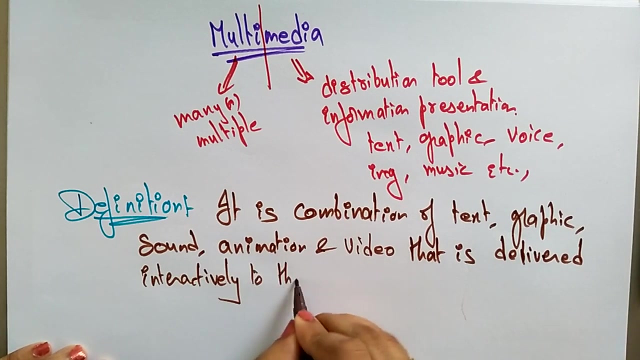 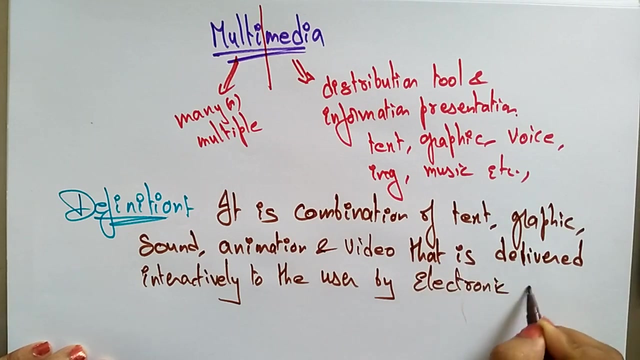 combination of a multimedia is a combination of text, graphic, sound or even animation, animation and video that is delivered interactively, That is delivered interactively to the user, to the user by electronic, by electronic or digitally manipulated means. digitally manipulated means so that you call it as multimedia. So this is the definition of multimedia. 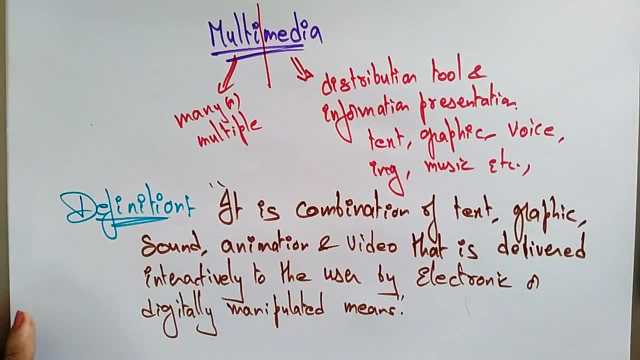 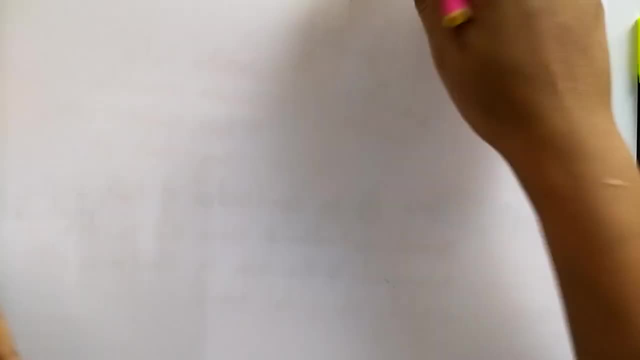 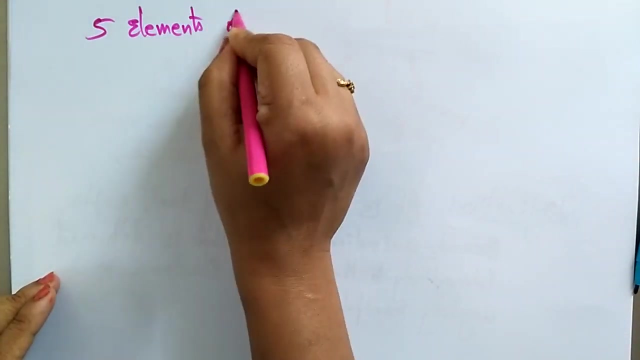 So, just, it is a combination of all things like text, graphic, voice, images, animation, sound and video, So which is delivered interactively to the users by electronic and digitally manipulated devices. There are total five elements of multimedia, are there? So? so, for whatever I said, those are the elements, the five elements of multimedia. So, what are the five elements of multimedia? 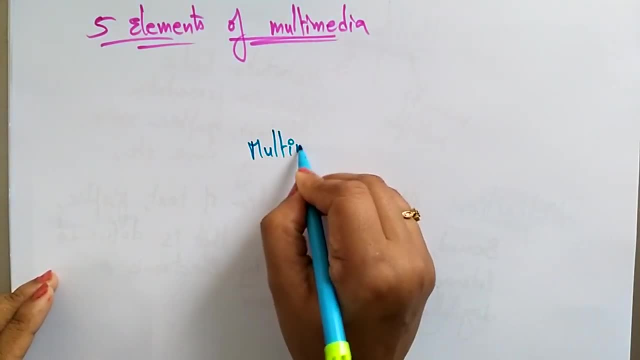 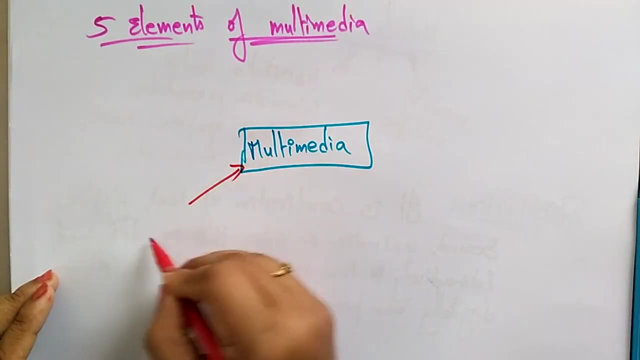 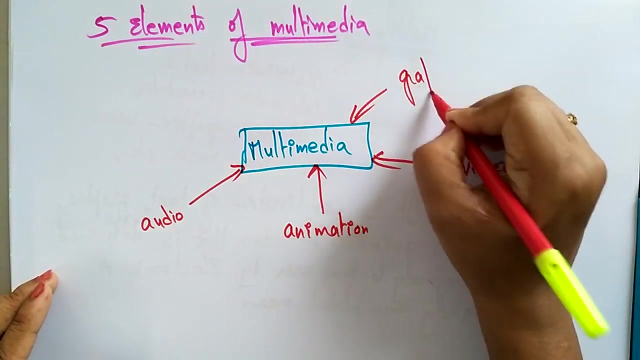 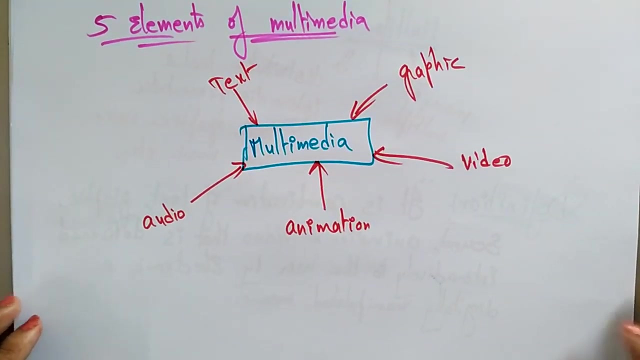 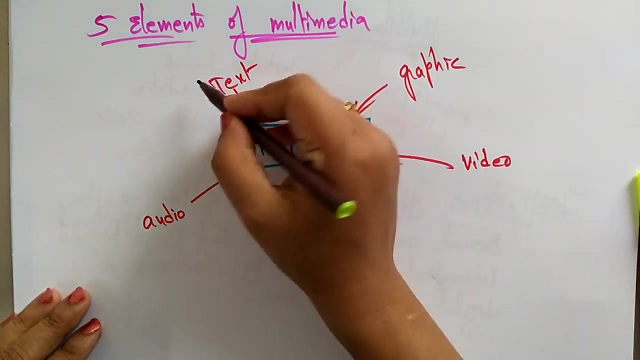 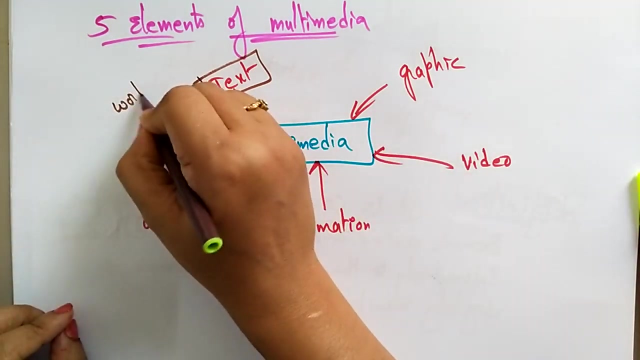 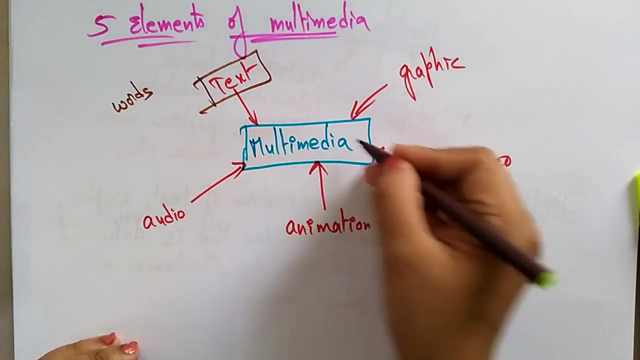 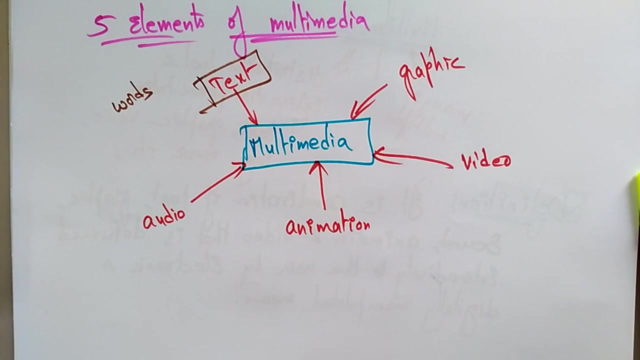 Multimedia. the five elements are audio, animation and video or even graphics, The most important in text. So these are the five elements of the multimedia: animation, video, graphic, text, audio. So let me discuss one by one. So what is a text here? Text, A text contains a word. So we already know that a text nothing but contains words, A words that express something. So I'm saying, okay, I'm writing here. So, whatever you're able to see the words, these are all the text. Okay, it contains words to express something. 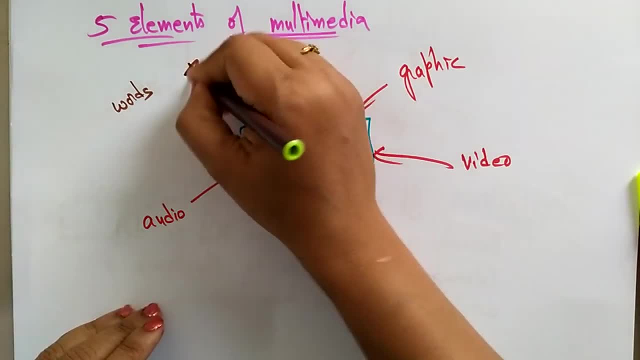 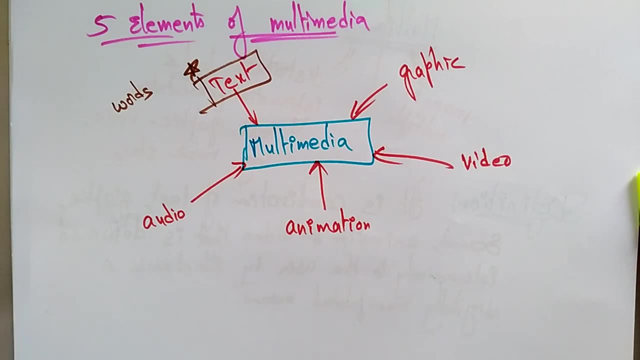 It is the most basic element of the multimedia. So text is the most basic element of the multimedia and it is used in the contents menus and navigation buttons and so on. And the next element of multimedia is let's take graphic Graphic. It's a 2D figure, 2D or 3D images, So that you call it as a graphics. It's just an illustrations. It could be produced manually. 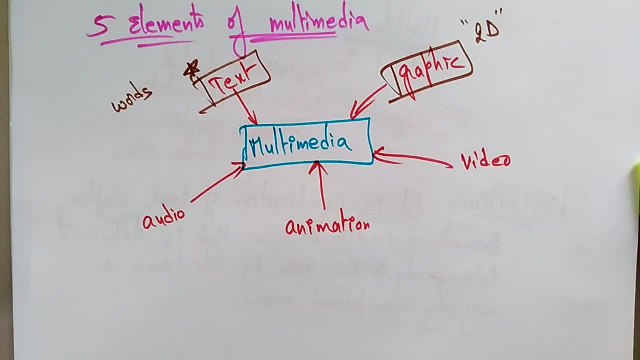 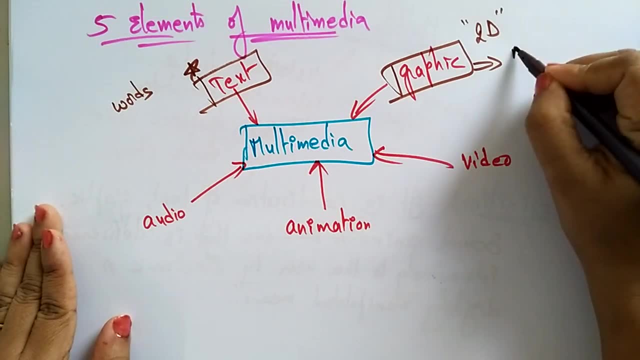 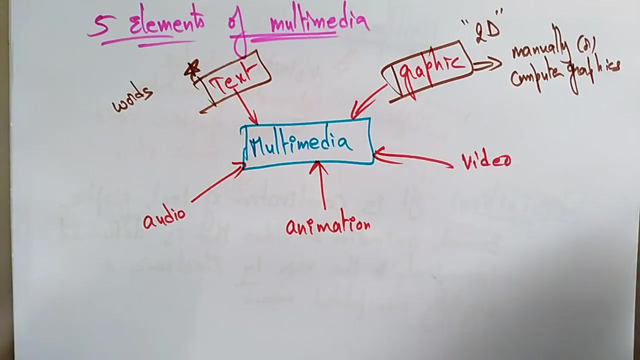 by drawing or painting or carving or by computer graphic technology. okay, so the graphic can be written by manually, it can be implemented manually or by using computer graphics, which is a technology. it's one of the technology and here the it is used in multimedia. so the main, this graphics. 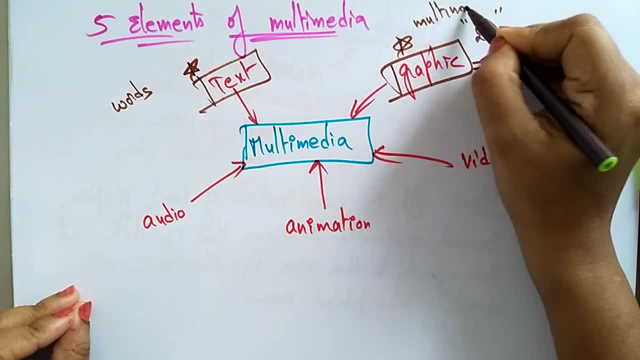 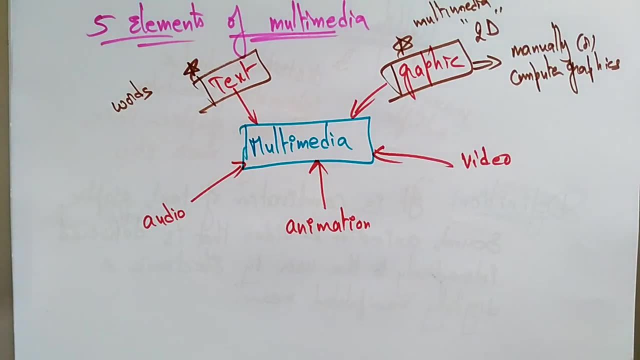 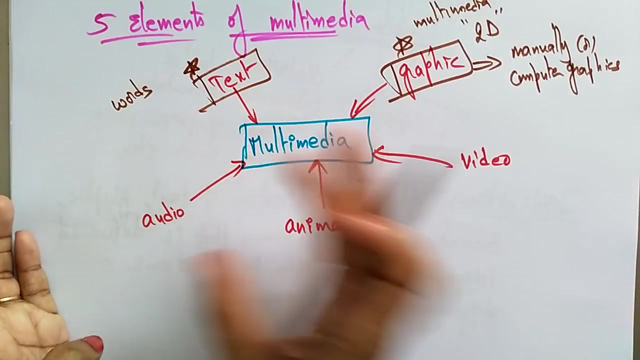 is used in multimedia environment: multimedia to show more clearly what a particular information is all about. the picture, okay. so, rather than seeing the text, if you see any image or a picture, it means the thousands of words, rather than seeing a particular information. these thousands of words can be represented in a single diagram, a single picture. so that is a graphic. 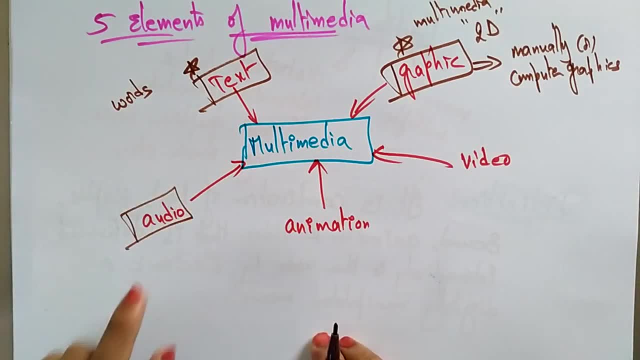 and let me take next audio audio. it is produced by vibrations. audio is produced by vibrations as per receipt perceived by the sense of the hearing. so aw, you can be here. it's just a vibrations which we can hear in multimedia. the audio could come in the form of a speech. it could 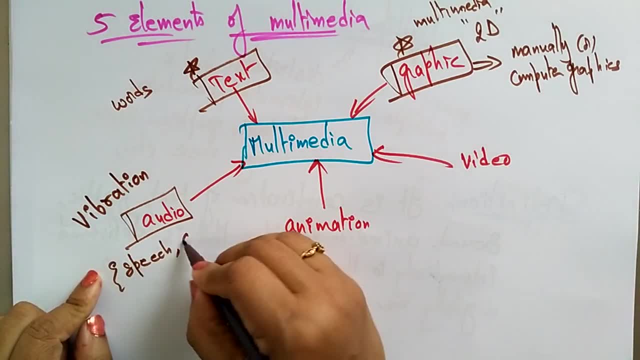 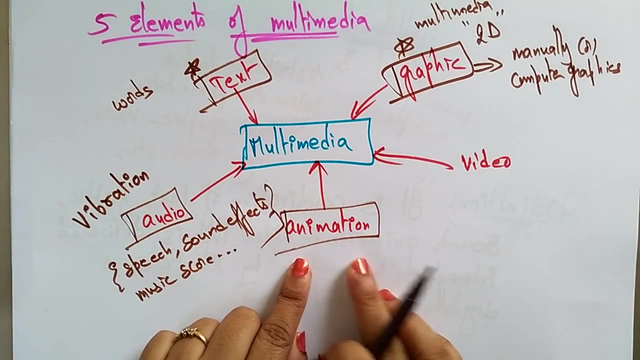 come in the form of a speech, or it can sound effects in the form of the audio, can be in the form of sound effects, or it can also come in the form of music score, and so on. now coming to the animation. animation. this animation is nothing but the illusion of emotion, illusion of motion, created by the consecutive displays of image, of.